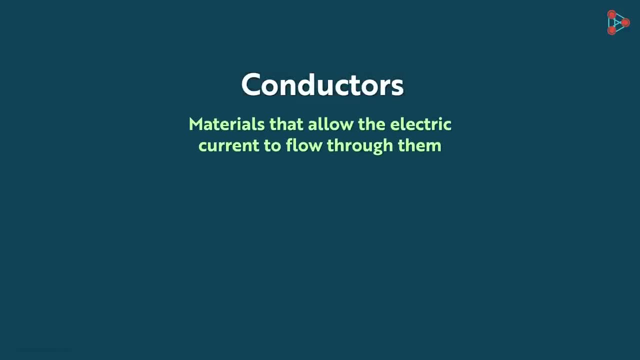 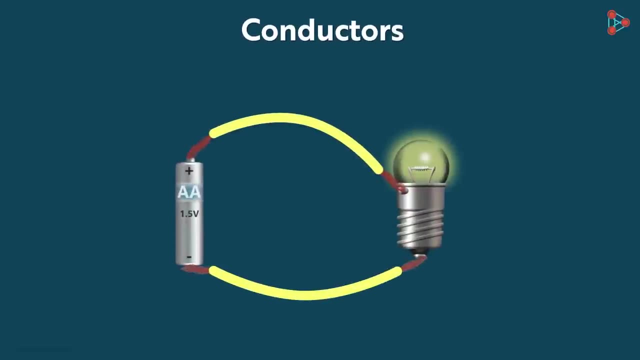 For simplicity, we will call them conductors. What are the examples of conductors? We have seen this simple circuit in the previous video. Here, a 1.5V cell is connected with a bulb, which can be between 3 to 4V, with the help of copper wires. 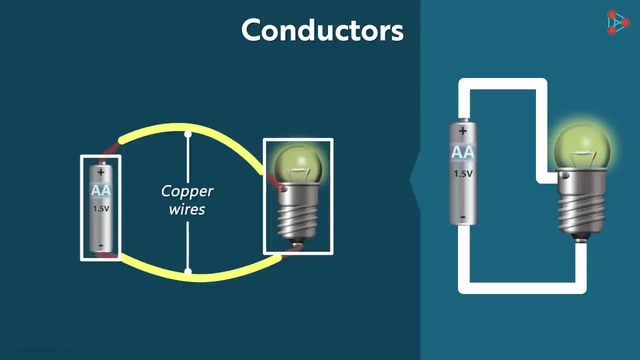 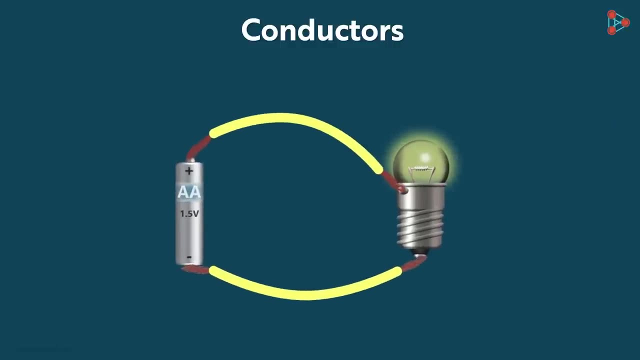 So here I told you that the movement of electrons is from the negative terminal of the cell to the positive terminal. But however, by convention, the direction of electric current is taken to be from the positive to the negative one. But how exactly is the current flowing in the circuit? 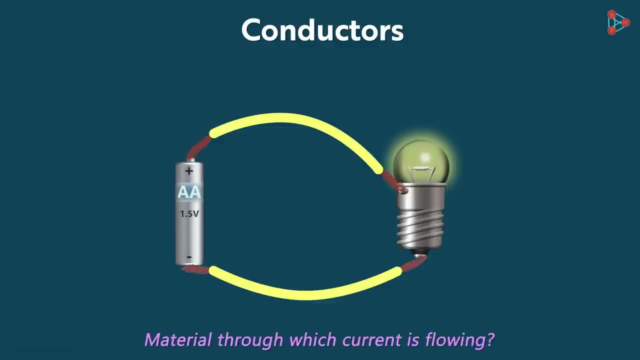 Or through which materials does it flow? What kind of material is this current flowing? Yes, it's the copper wires. Electric current is flowing through the copper wires from the positive to the negative terminal. So what can we conclude from this? We say that the copper is a conductor of electricity, since it allows the electricity to flow through it. 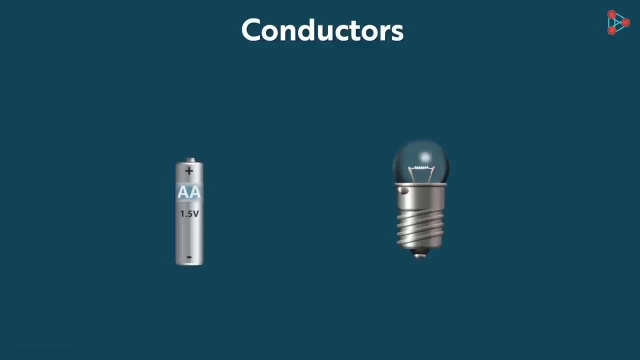 Now, instead of copper wires, what if we use pieces of threads in the circuit? Will the bulb glow in that case? No, it won't. Why, Because the electric current cannot flow through a piece of thread. Such materials are called insulators. 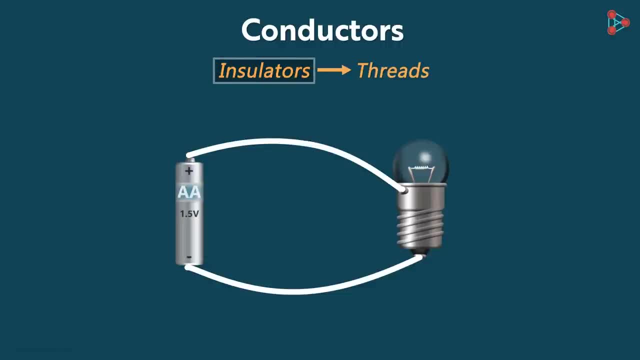 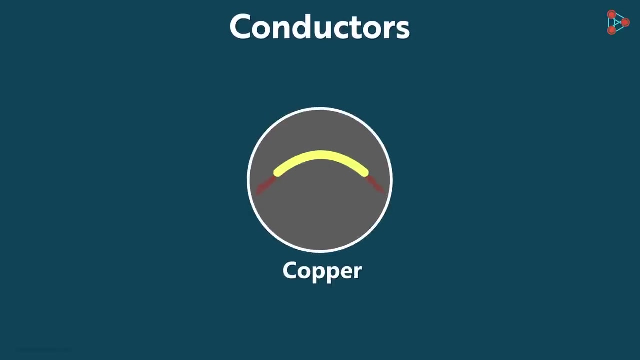 So how do we define this term? Give it a try. These are the materials which do not allow the electric current to flow through them. Let's study a bit about conductors first. Besides copper, what are the other materials that conduct electricity? 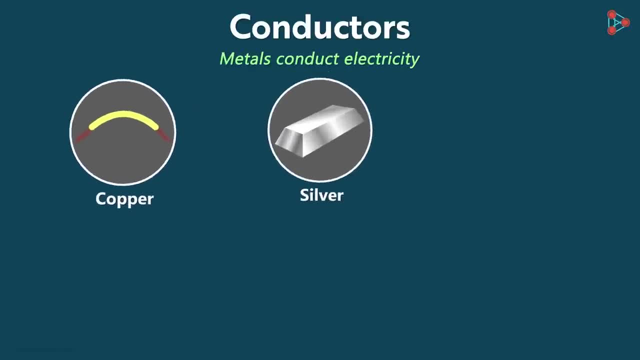 Almost all metals conduct electricity. Almost all metals conduct electricity. Almost all metals conduct electricity. SILVER, GOLD, ALUMENIUM, IRON AND MERCURY. Almost all metals conduct electricity. Silver, gold, aluminium, iron and mercury are a few other examples of metals. 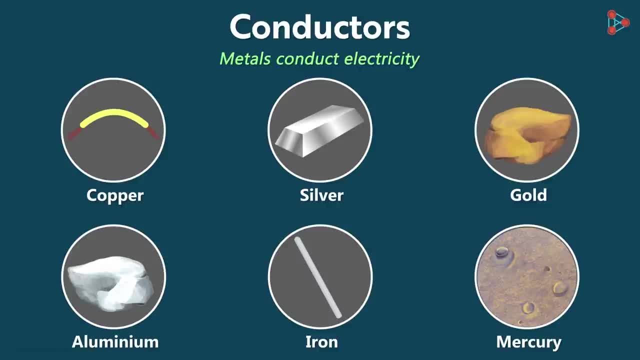 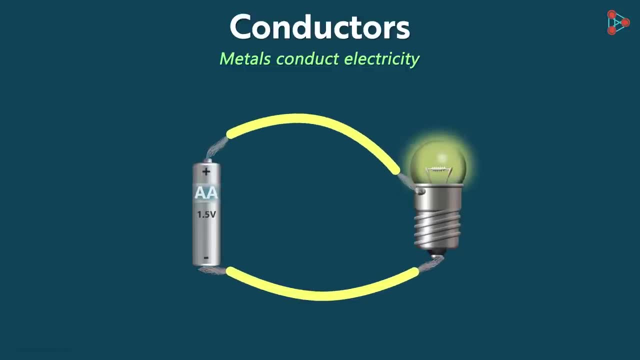 that conducts electric current. If you replace copper wires in our circuit with aluminium once, then you will find that the bulb is from the Perm extremity. This proves that aluminium allows electric current to flow through it. In fact, this area of the bulb is itself made up of metal. 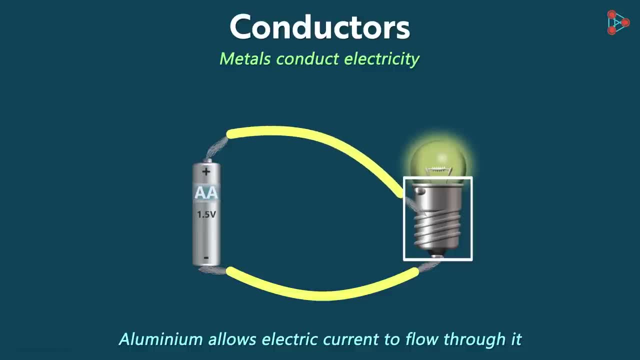 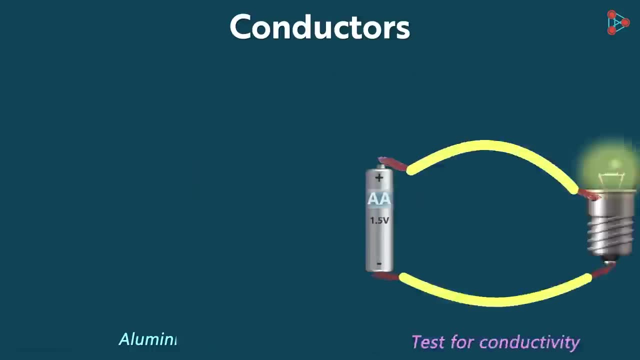 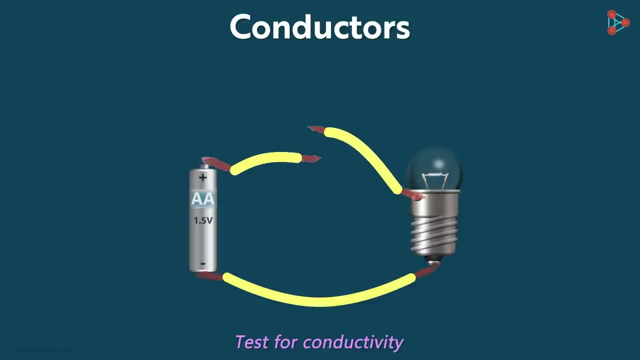 Hence, if we connect the wire anywhere in this region region, the bulb will still glow. It transfers the electricity to the terminal of the bulb and inside We can actually test any object for conductivity. Break this circuit up from anywhere by cutting the copper wire.